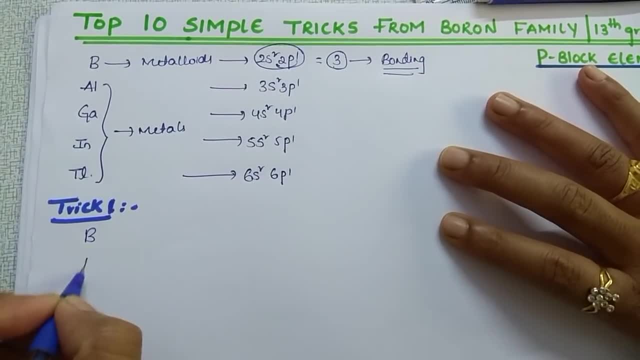 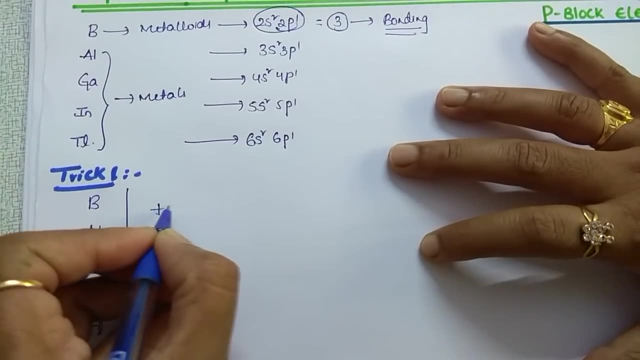 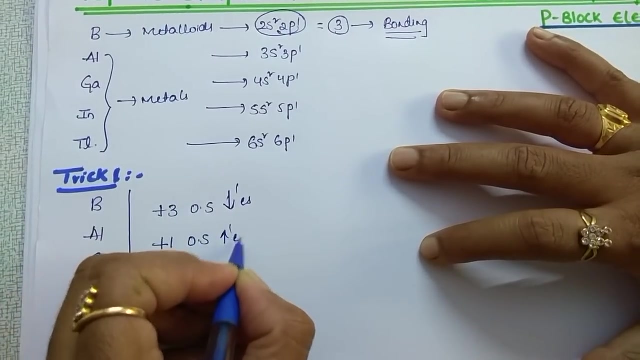 3 is the oxidation state. boron, aluminium, gallium, indium, thallium. important thing is: down the group, plus 3 oxidation state decreases and plus 1 oxidation state increases. this is very, very important students. down the group, what happens? plus 3 oxidation state decreases and. 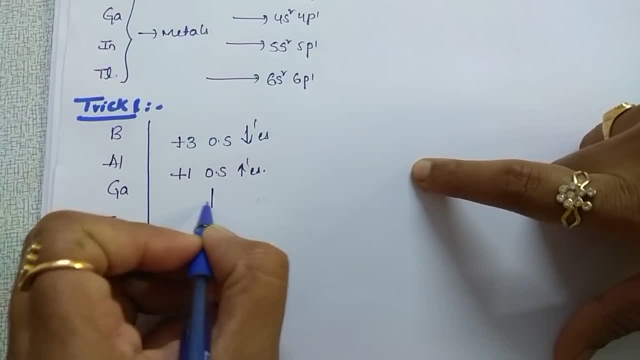 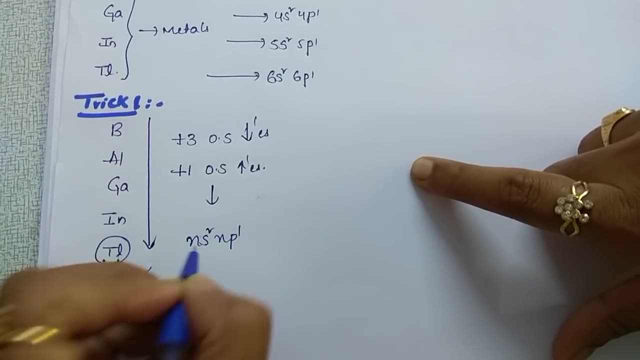 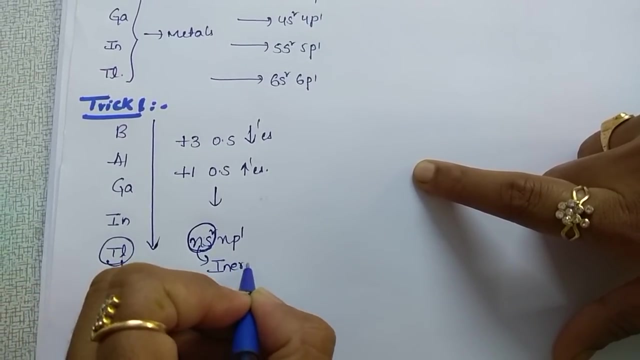 plus 1, oxidation state increases. reason is actually here. what happens is in the case of down element like thallium, general electronic configuration is ns2, np1 right. these two electrons won't involve in bond participation. they becomes inert, and this one we call it as inert pair effect. 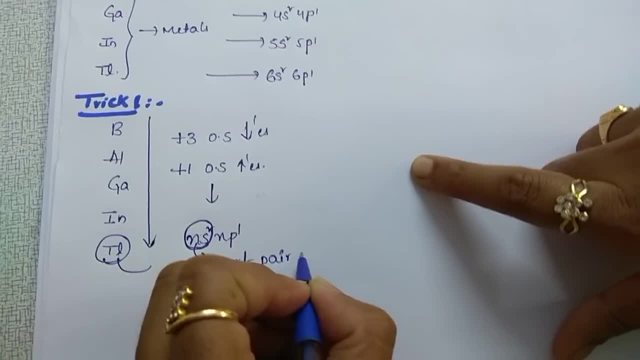 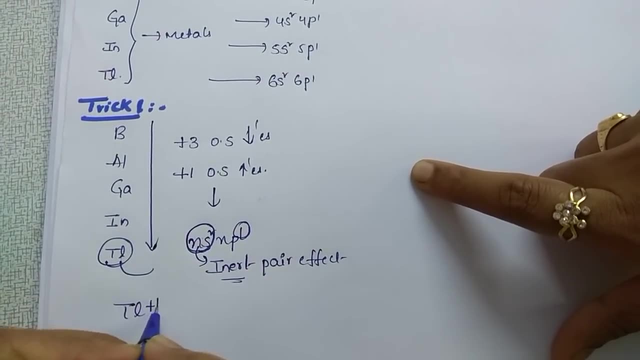 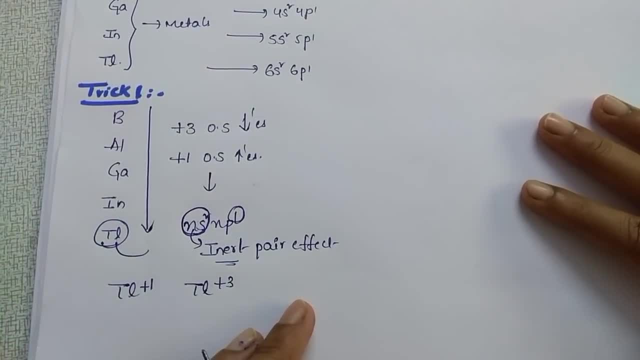 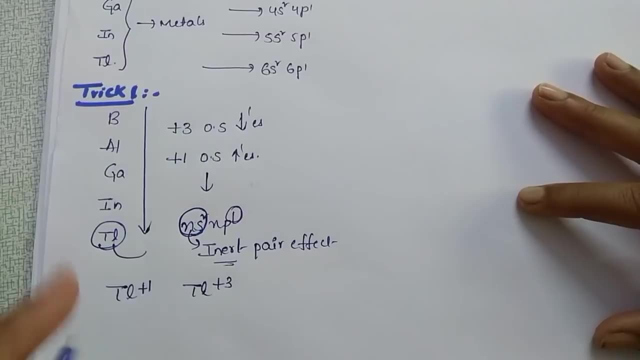 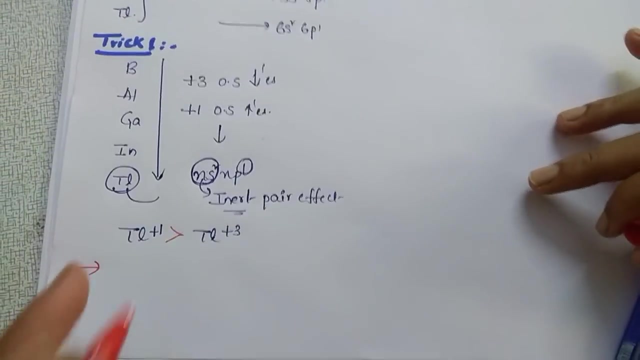 and tl plus 3, which is more most stable oxidation state for thallium. thallium belongs to group number 3, so plus 3- if you mark it will be wrong, it is plus 1 state is more stable. this is due to inert pair effect. and one more question i'll cover here: out of tl cl 3 and tl cl and tl cl 3, which is 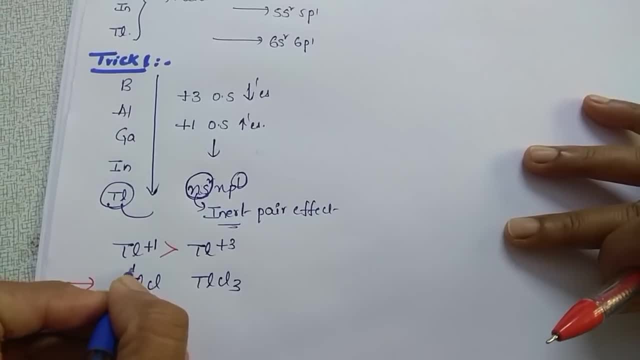 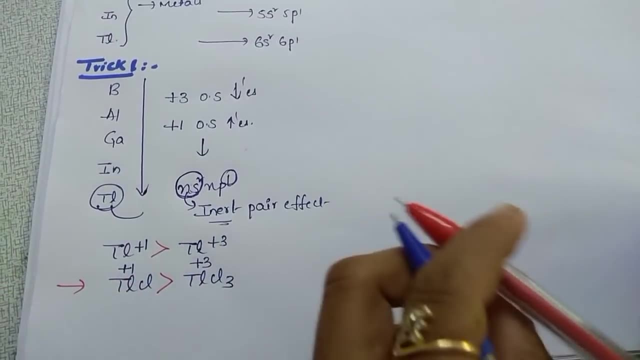 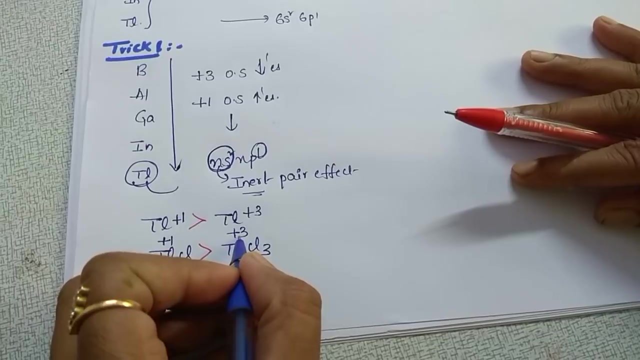 more stable. same question another way: in tl cl thallium is in plus 1 and in tl cl 3, thallium is in plus 3. so which is more stable? tl cl is more stable. and one more question is: in these two, which one acts as an good oxidizing agent? then just, it is in thallium, is in plus 3 state. it will actually. 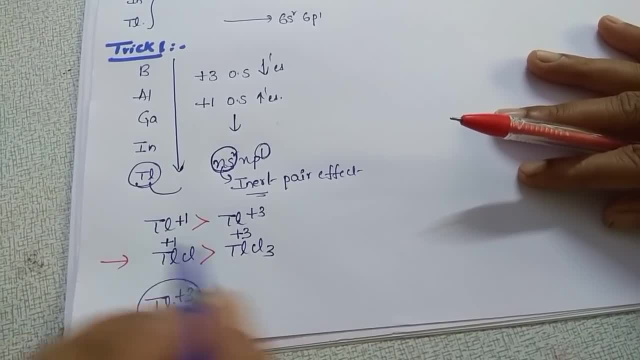 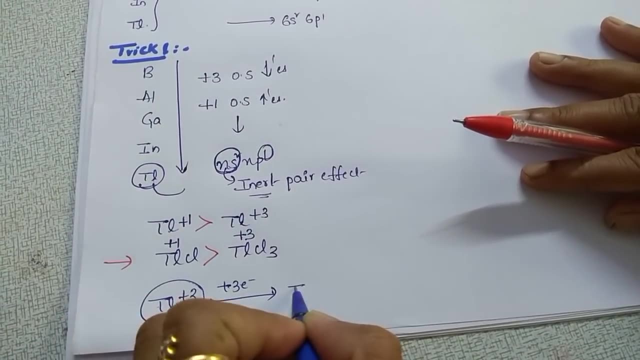 generally it is unstable in this state. it tries to convert into plus 1 state because thallium is stable. in plus 1 it gains 3 and plus 1 state. so it will try to convert into plus 1 state because electrons and it converts into sorry 2 electrons and it converts into thallium plus 1. so it is. 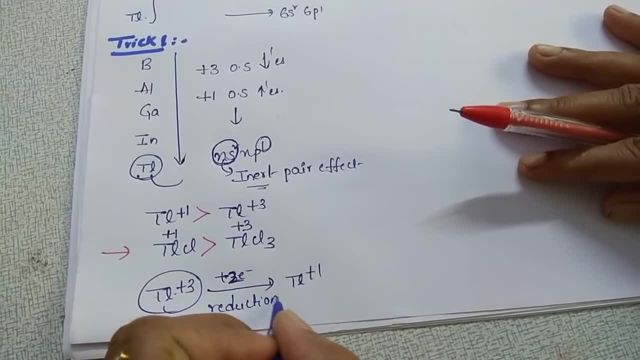 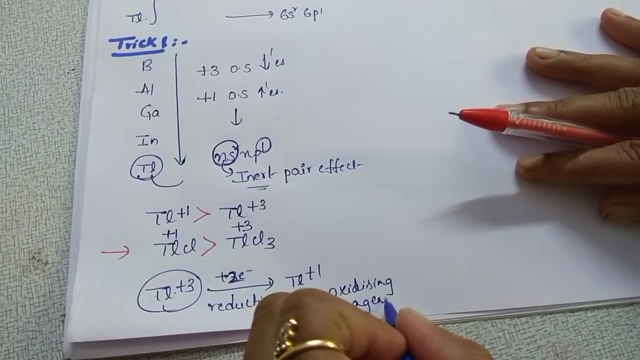 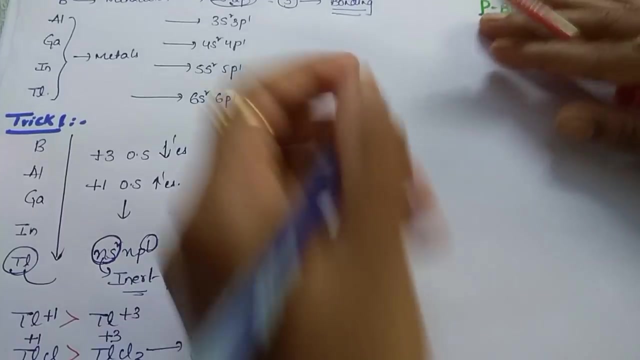 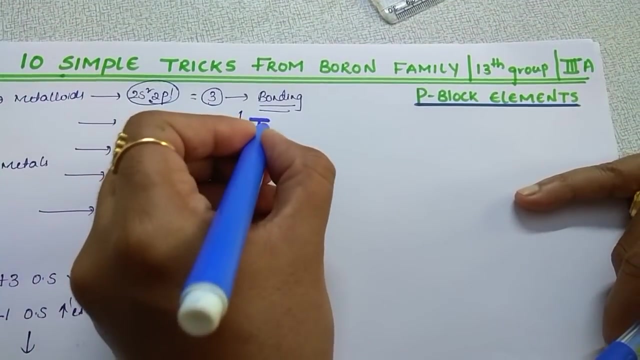 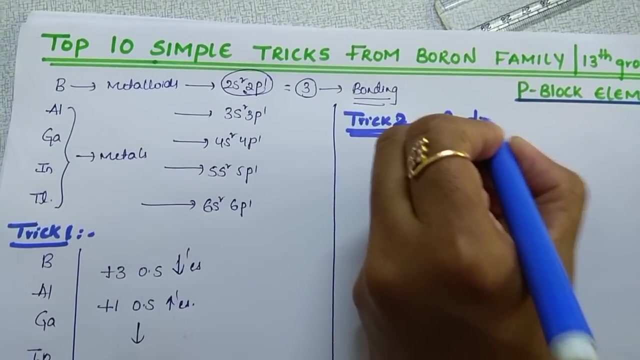 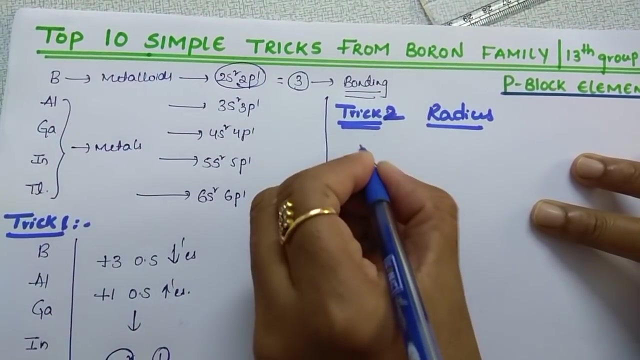 undergoing reduction. whenever it is undergoing reduction, it acts as oxidizing agent. oxidizing agent. so tl cl 3 is good oxidizing agent. this is our trick one. here we covered three kinds of questions. next, trick number two. this trick is regarding regarding radius. generally down the group, what happens is number of shells increases. whenever number of shells 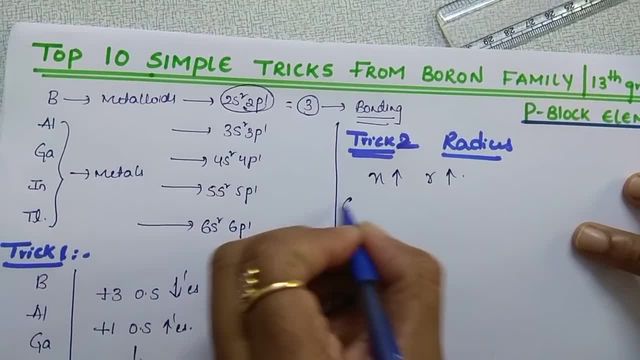 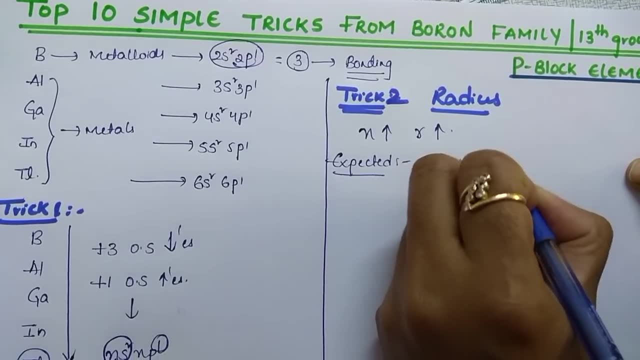 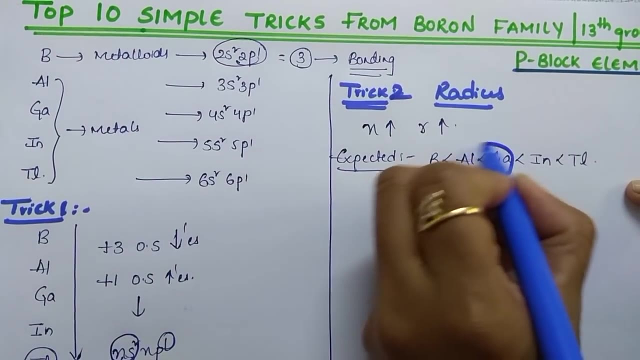 increases. radius also increases expected. so expected radius is: boron, aluminium, gallium, indium, thallium- down the group radius is expected. so down the group radius is expected. so down the group increases. this is the expected radius, but keep it in mind this is the exceptional case. 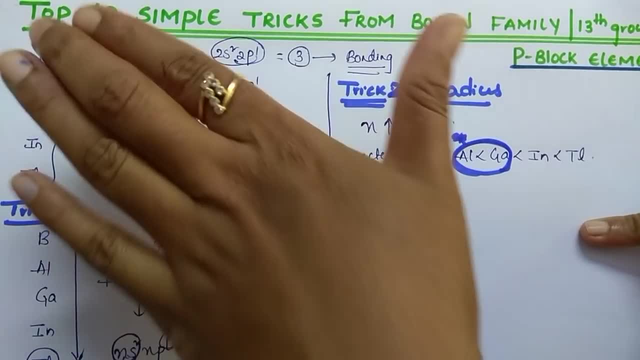 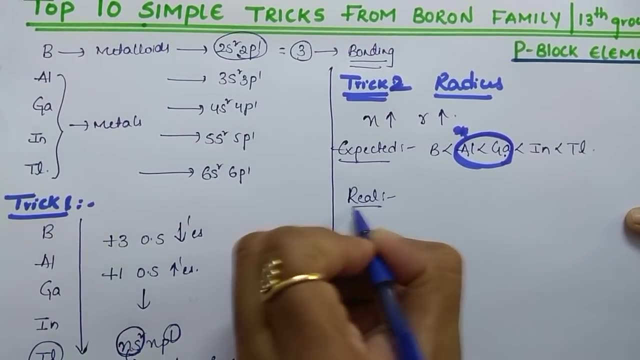 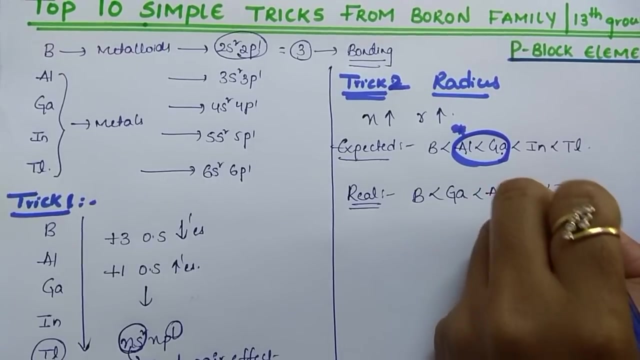 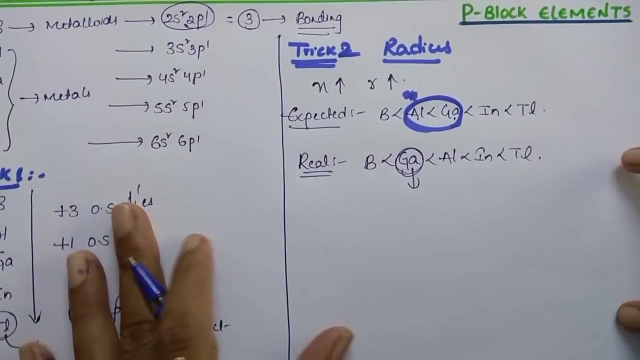 this is the common questions which is asking from boron family, gallium and aluminium. the real experimental order is boron. next gallium comes here. aluminium, indium, talium. gallium is having less atomic radii when compared to the aluminium. the reason for this is gallium is having 3d. 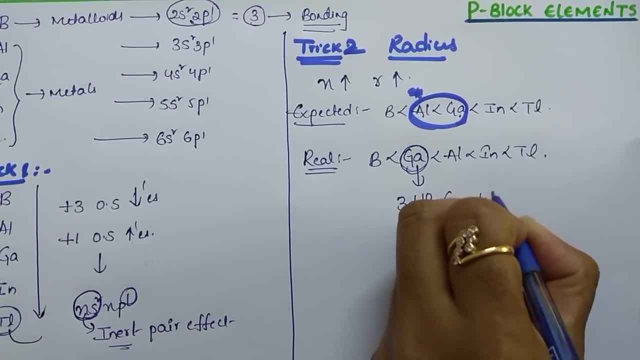 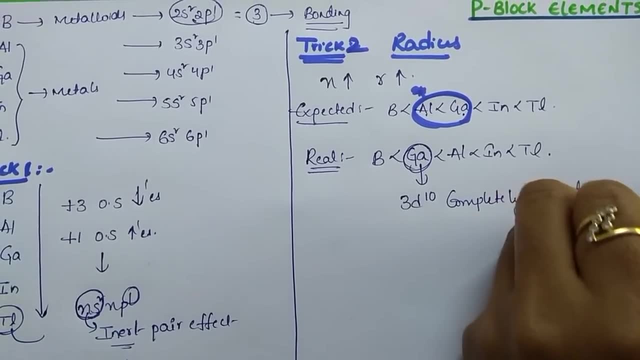 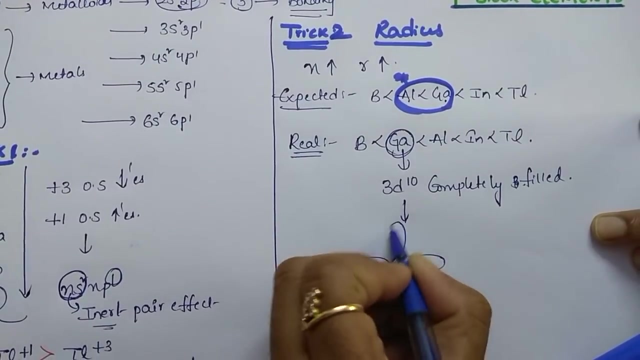 completely filled 3d subshell whenever it is having completely filled. 3d subshell is completely filled whenever it is completely filled. what happens is: we know that d orbitals are diffused. their lobes are diffused- diffused in the sense large. diffused means large. 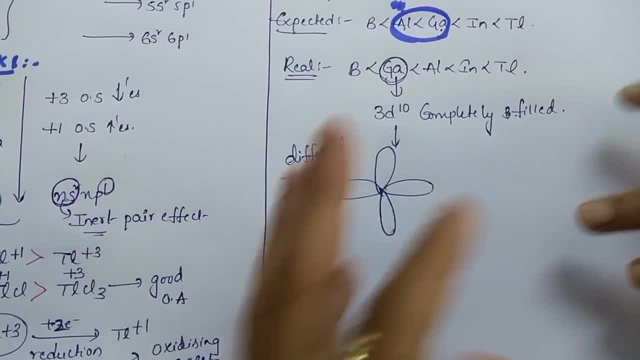 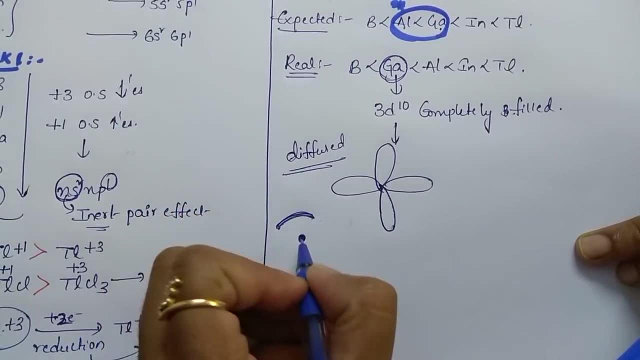 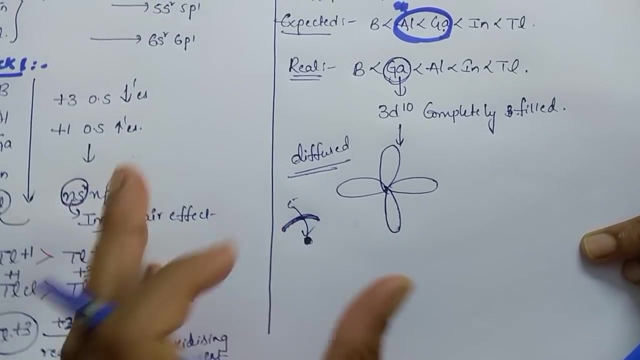 clear. whenever lobes are large, electrons are. electrons are free to move. suppose here is a nucleus, here electrons are present. what happens is these electrons acts like a screen so that this nucleus cannot attract the valential electrons. then size will increase. here these electrons acts like a. 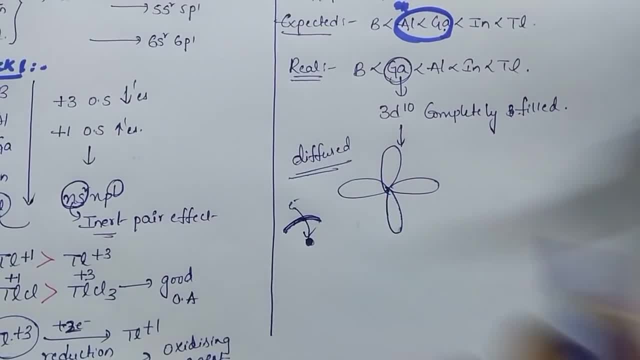 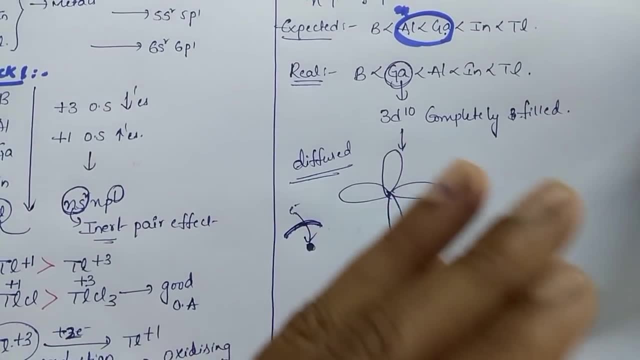 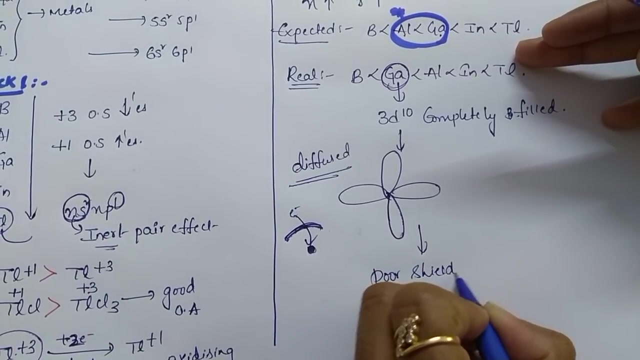 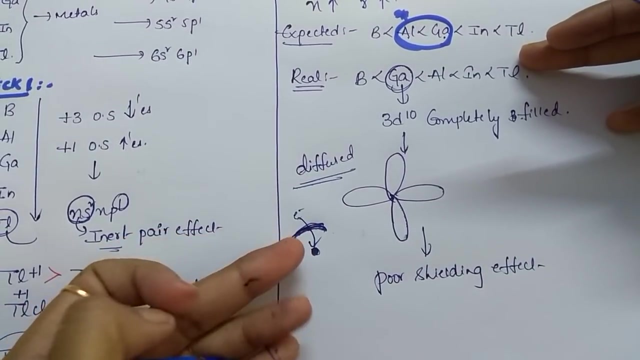 screen. but in the case of d orbitals what happens is they, their lobes are diffused, their lobes are very large. then what happens? they cannot acts like a screen, they show poor shielding effect whenever they. they show poor shielding effect, then nucleus these electrons cannot acts like a screen, then this nucleus attracts these. 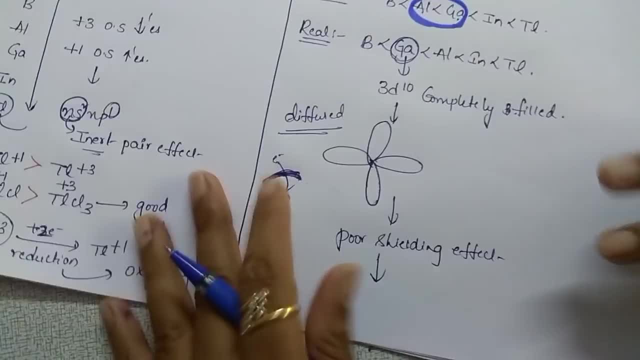 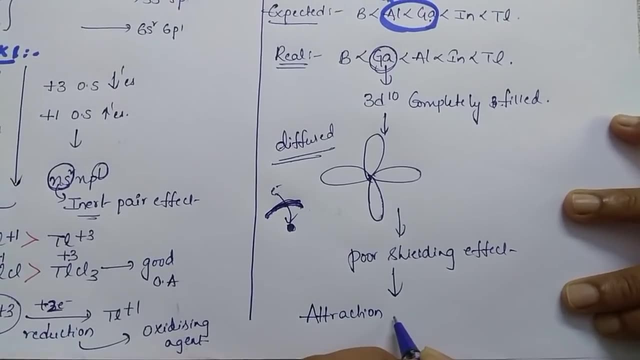 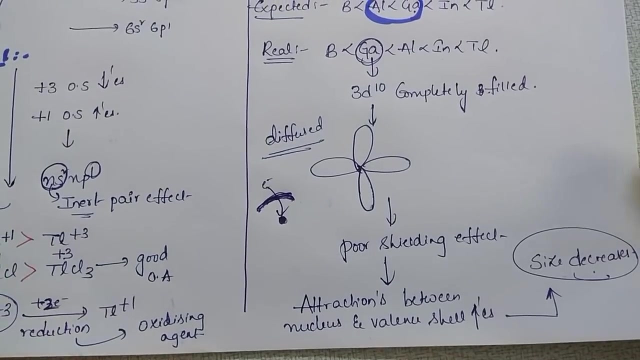 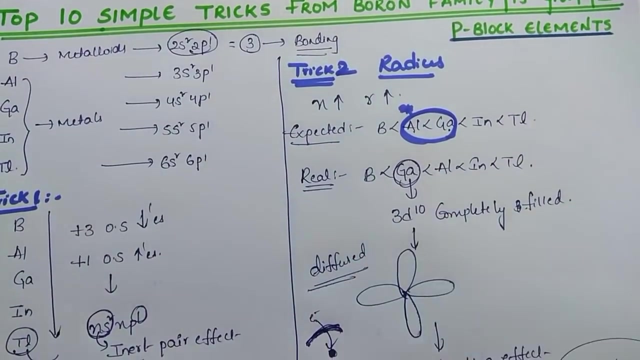 valential electrons easily, so that attraction between, attraction between nucleus and valential, increases attractions between between. whenever attractions between nucleus and valential increases, size decreases. that is the reason aluminum and gallium gallium should have more radius, but aluminum is having more radius than the gallium. 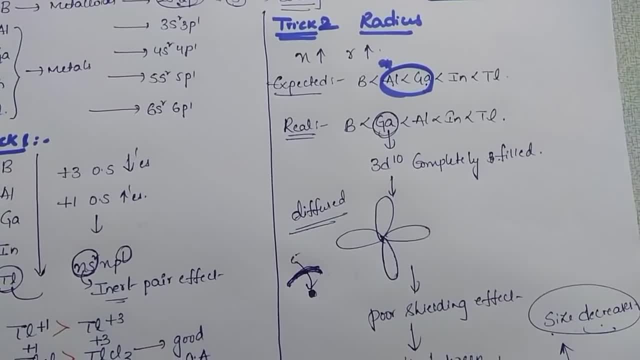 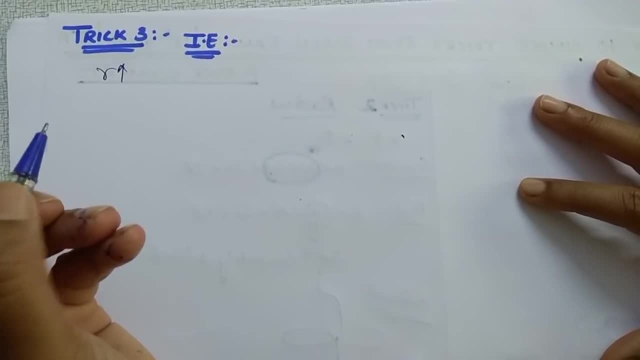 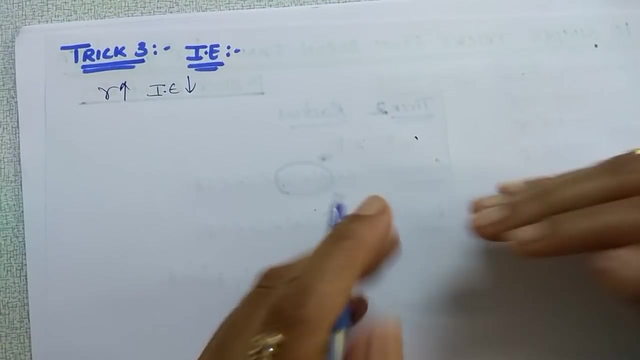 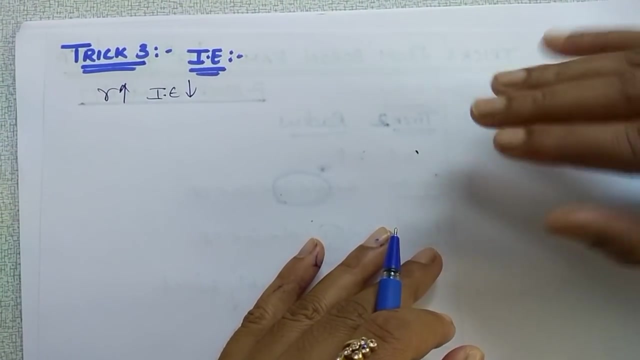 trick number three. this trick is regarding ionization energy generally. whenever radius increases down the group, then ionization energy will be reduced so that it will be more. ionization energy decreases because whenever size increases, it means that the distance between the nucleus and the valential increases. whenever it increases, whenever number of shells are more and 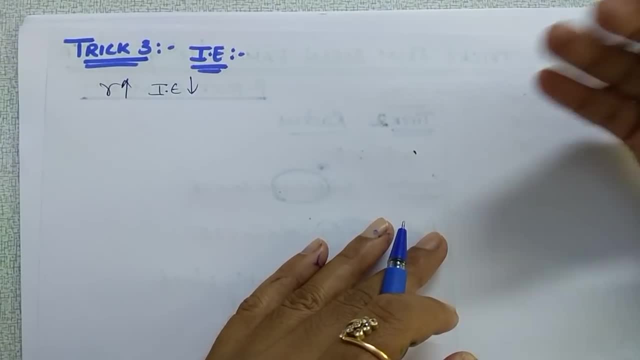 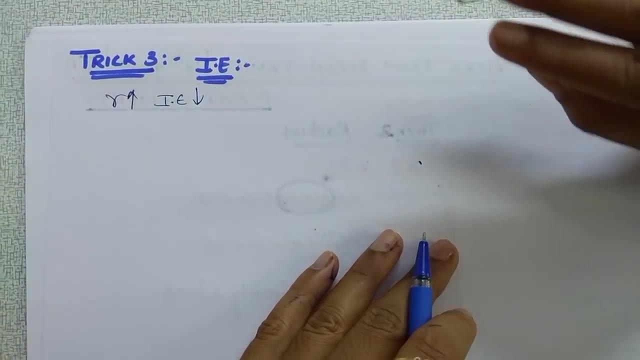 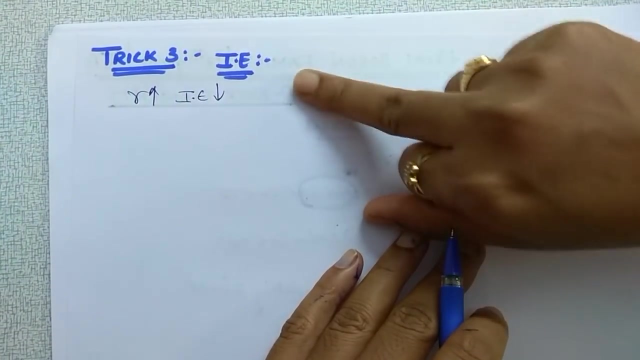 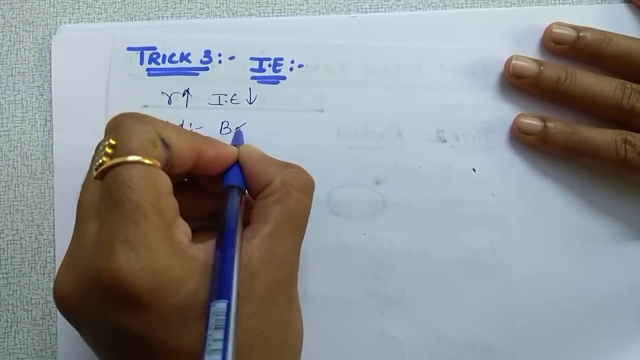 the attractions between the nucleus and the valential electron is less, then distance increases. whenever distance is increases and nucleus effect on valence electron is very less, so that it is very easy to remove the valential electron, then that is the reason ionization energy decreases. so the expected order is expected one is boron, aluminum, gallium, indium, thallium. here i 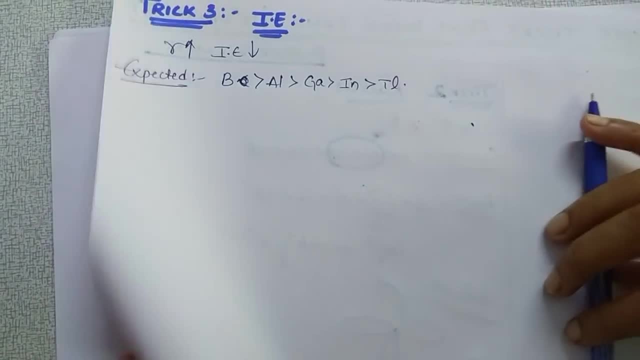 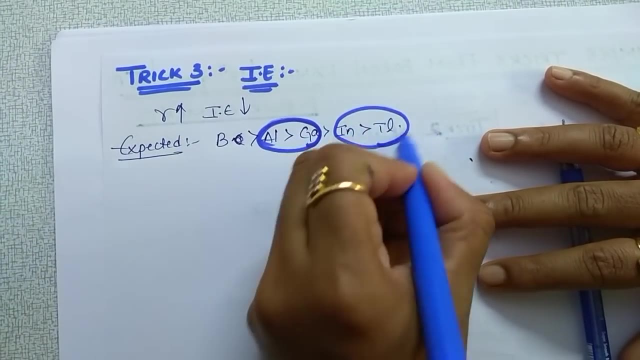 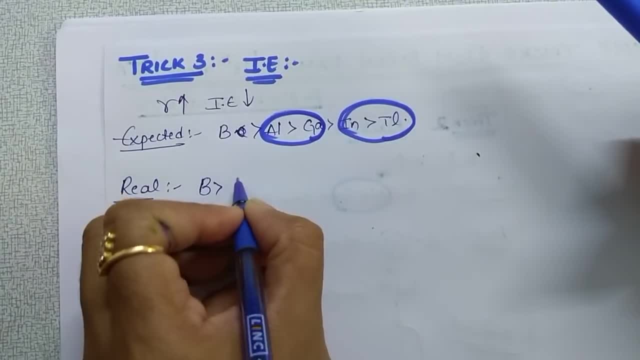 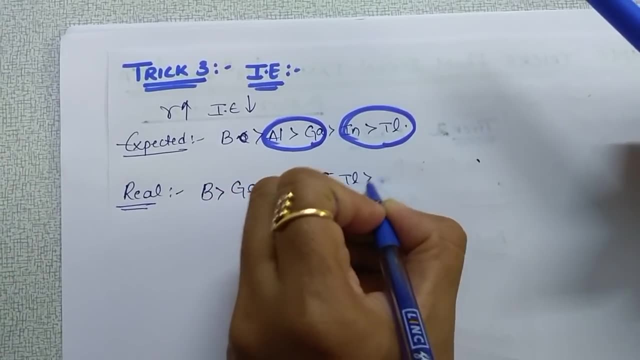 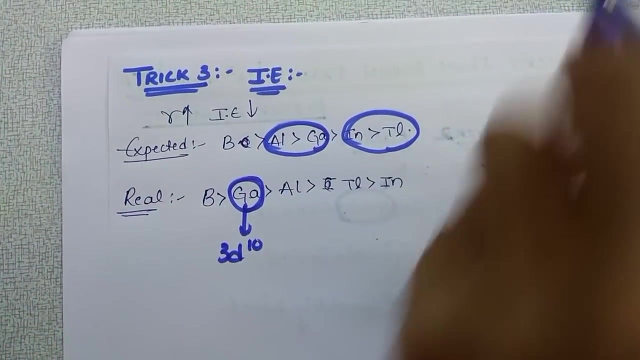 experimental trend is boron first, then gallium is having more ionization energy than aluminum, then indium is having- sorry, thallium is having more ionization energy than indium. actually, the reason for this is gallium is having 3d 10, completely filled 3d 10, and thallium is having 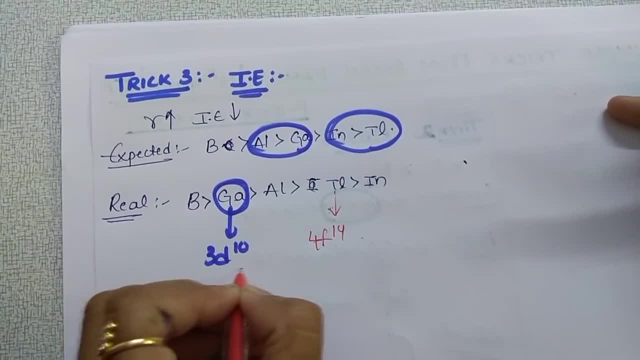 completely filled 4f subshell. whenever this 3d and 4f subshells are filled, actually 4f. if you observe the size of the subshells, it is actually 4f subshells. it is actually 4f subshells. 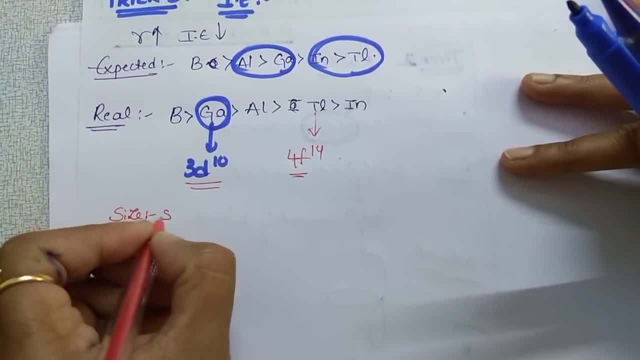 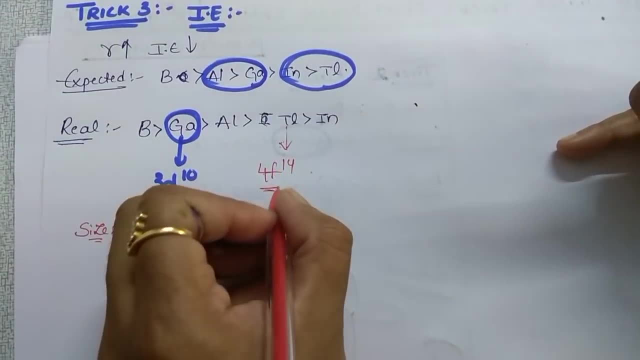 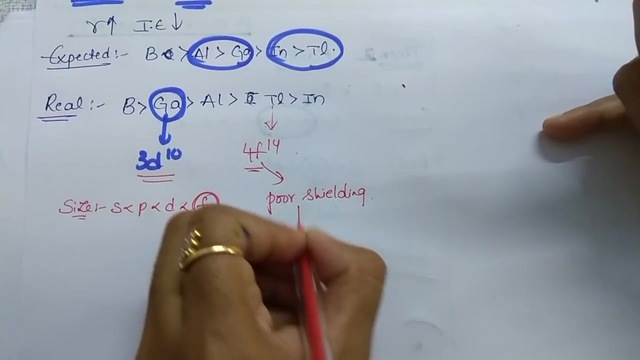 if you observe the size of the orbitals, what happens is s, p, d and f? f. also lobe lobes are diffused, large lobes, then these acts as a pore screening. they show pore shielding. whenever they show pore shielding, attraction between nucleus and valence electrons increases attractions. 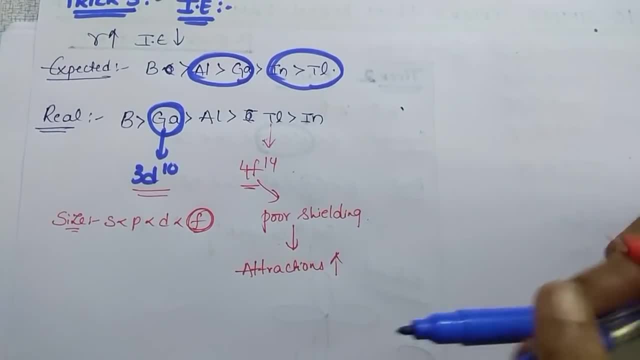 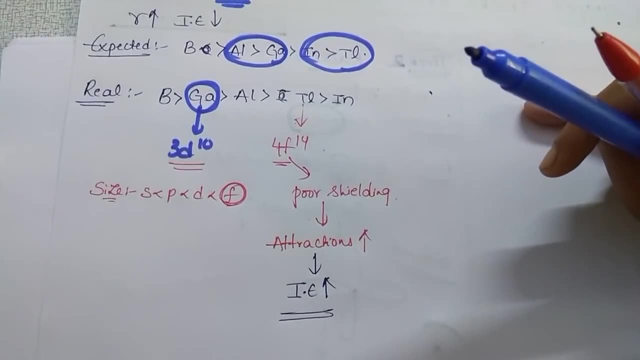 increases, whenever attractions between nucleus and electron increases, then it is difficult to remove the valence electron and it is difficult to remove the valence electron and it is difficult. ionization energy will be more. that is the reason thallium ionization energy is more than the. 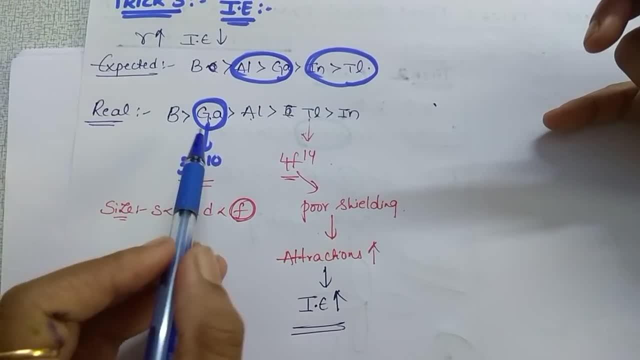 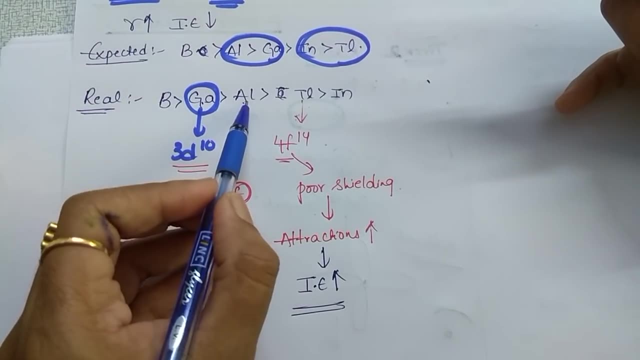 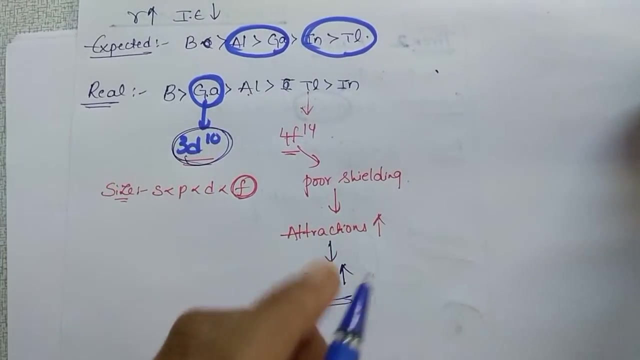 indium and gallium and aluminum we already discussed. a size effect is there and automatically ionization energy. also more for the gallium when compared to the aluminum due to the completely filled d orbitals and it shows pore shielding attractions increases. and thus what to say? 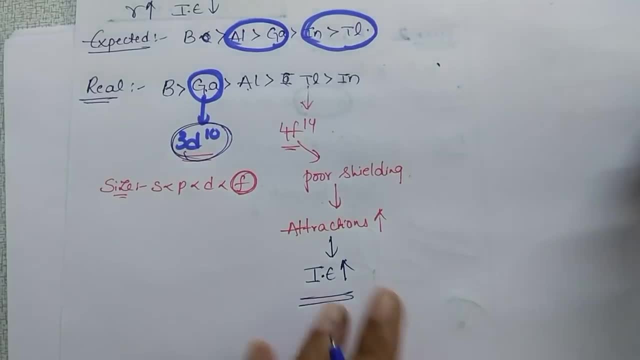 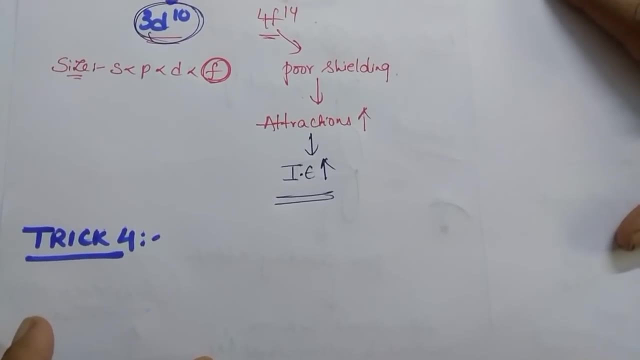 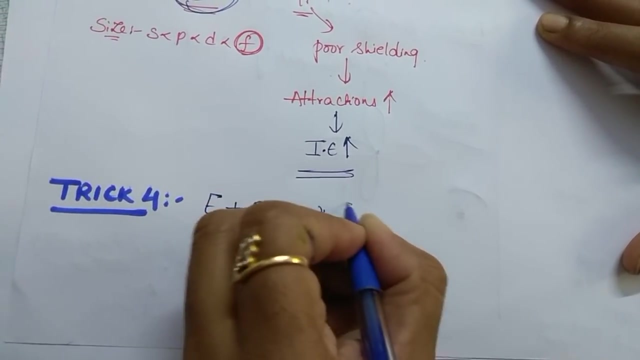 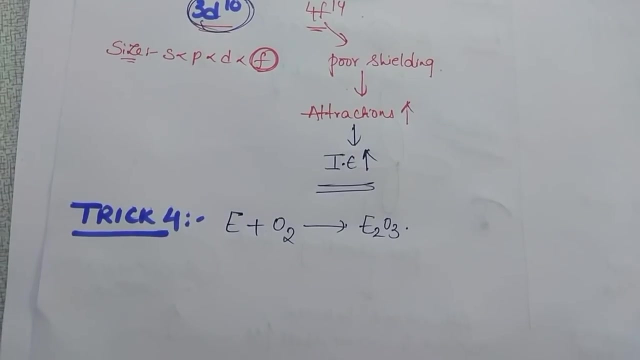 attraction increases, it is very difficult to remove the electron number four. whenever these elements reacts with the air then like, suppose, if it is reacting with oxygen then it forms oxides like e2o3, generally reactivity: i'll tell you in you easily, you can do the reactivity. size increases- students see here. size increases, then what happens is reactivity. 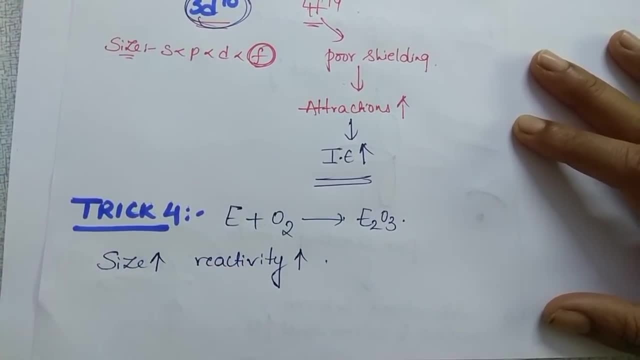 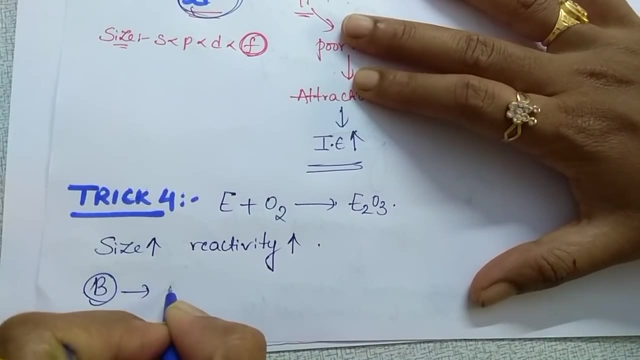 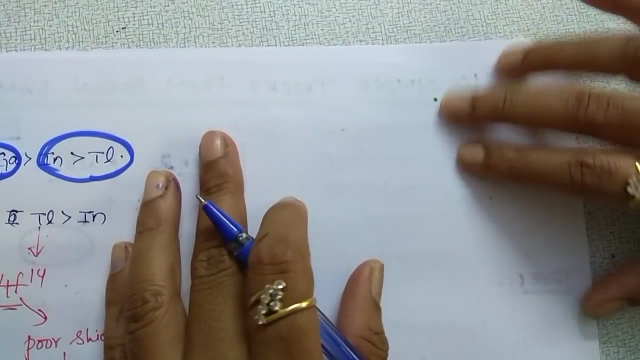 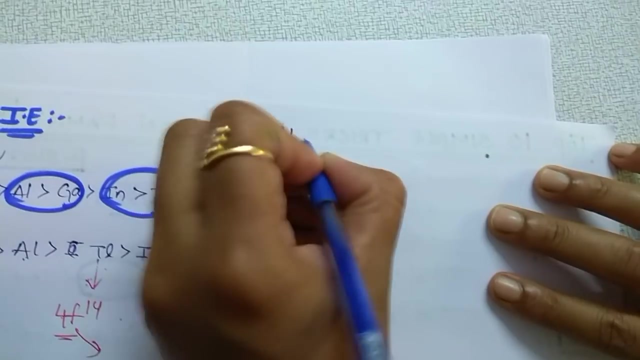 of the element increases. what happens? size increases, then reactivity of the element increases, then you can say: boron is small size, so boron is almost non-reactive. and now i'm going to discuss about this, aluminium, which is most important. questions are: aluminium reacts with oxygen and it forms al2o3. this is very important reaction, see: 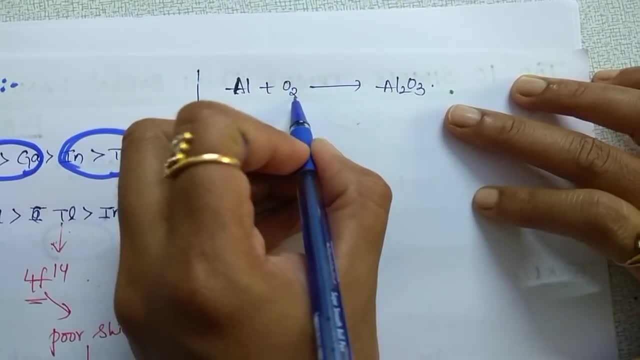 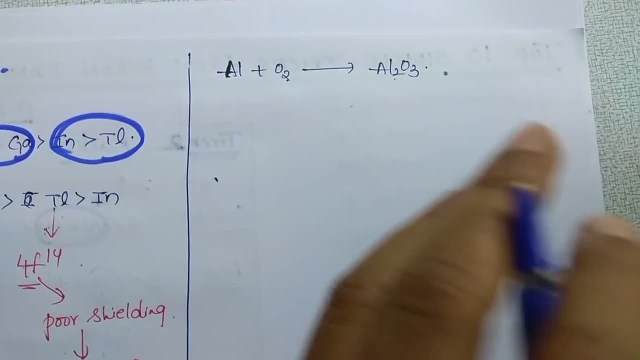 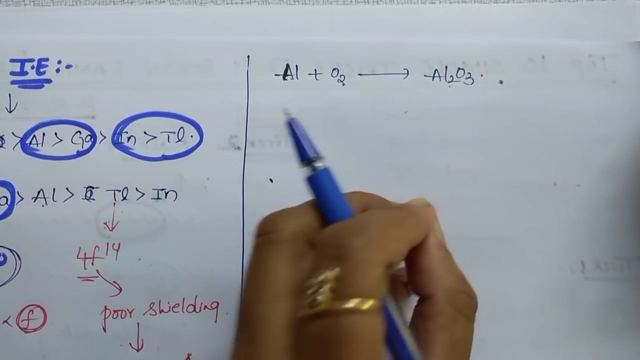 you get, you get, you get questions from this. whenever aluminium reacts with oxygen, it forms al2o3. this aluminium also, you can say almost less reactive, but it is also non-reactive. but it is less reactive, we can say its reactivity is little more when compared to boron. actually, the reason for its non-reactivity is aluminium first. 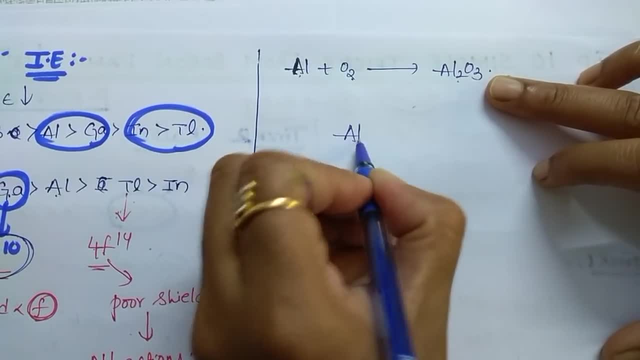 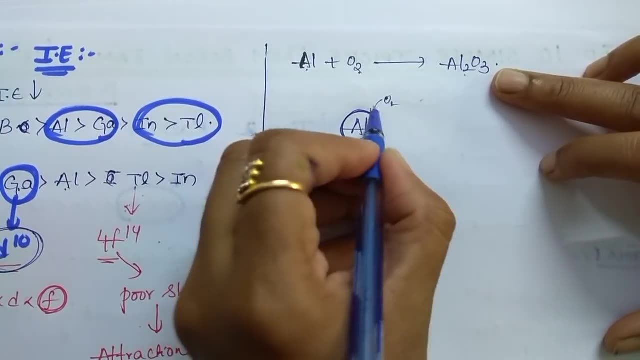 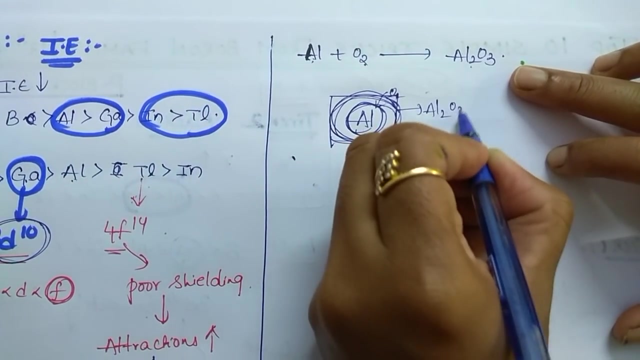 reacts with oxygen and it forms al2o3. this al2o3- suppose this is a metal it reacts with when it is exposed to air. it reacts with oxygen and it forms al2o3. this al2o3 forms like a layer around aluminium. this is a layer of al2o3. once this layer of al2o3 is formed, it stops a further reaction of. 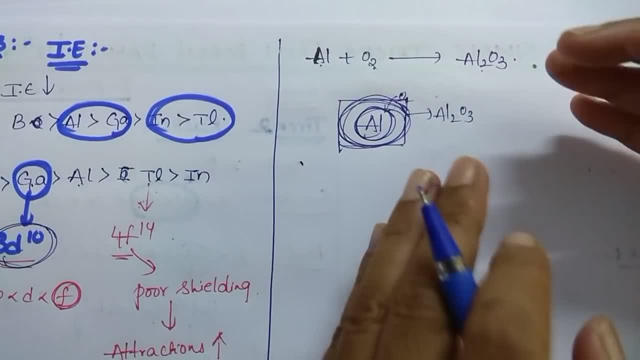 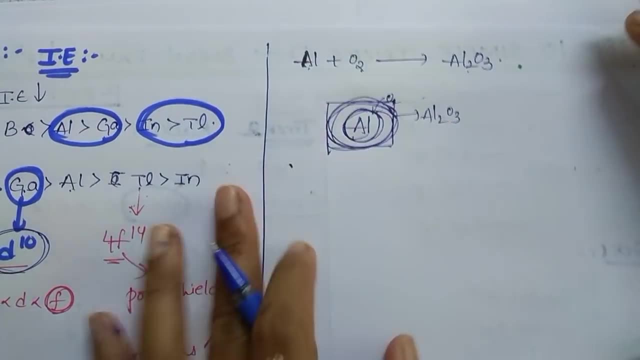 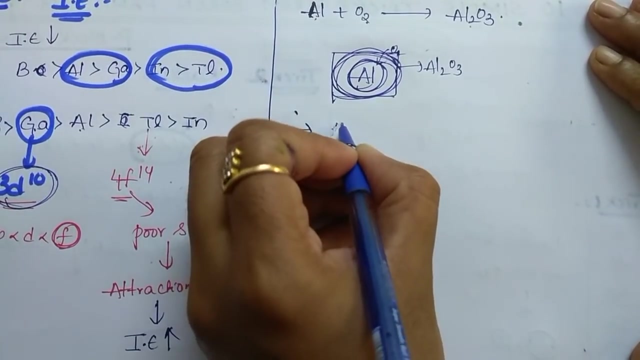 this aluminium with the oxygen clear. this is called as protective layer of al2o3, which protects this further reaction of aluminium with oxygen and whatever the oxides are there here. i'll cover one more question that suppose if you see b2o3, boron won't react with oxygen, but at high temperatures. 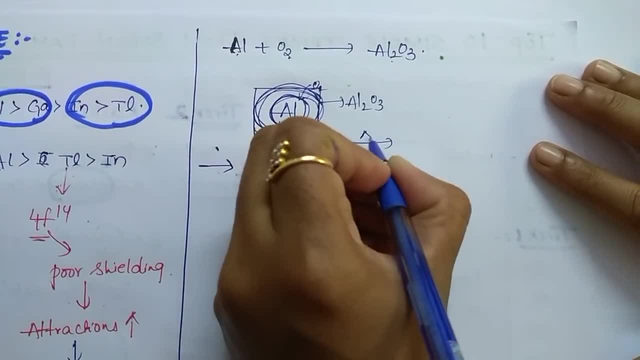 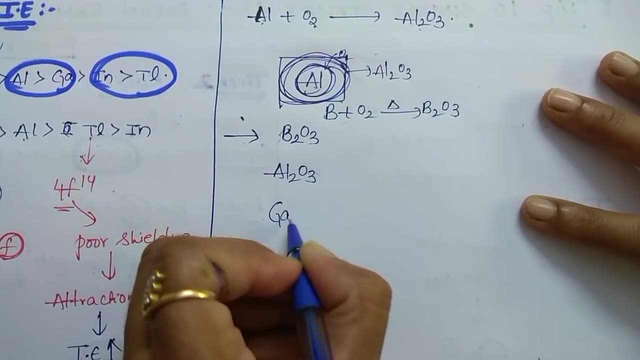 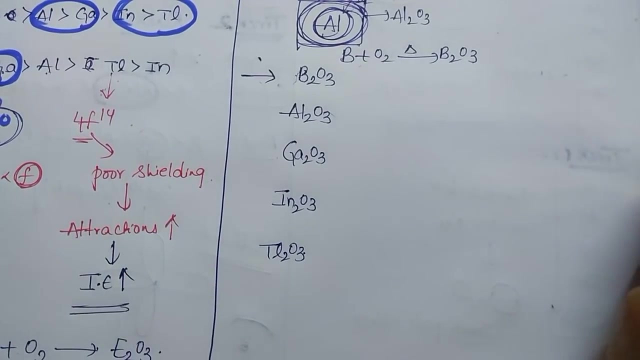 boron reacts with oxygen and it forms b2o3 right out of this b2o3, al2o3, ga2o3, in2o3, tl2o3. they ask the nature of the oxides generally. b2o3, boron reacts with oxygen and it forms al2o3. this al2o3. boron oxide, or boron. its name is sesquioxide. i'll discuss about that trick. also, b2o3, it is acidic oxide. why it is acidic oxide? because whenever b2o3 it reacts with water, generally it reacts with water. b2o3 reacts with water, then it forms boric acid because of the formation of this acidic compound b2o3 is decided as it is an acidic oxide, l2o3. generally it reacts with both acids as well as a basis that is called as amphoteric. i'm going to discuss these reactions also. amphoteric and the remaining three oxides are basic. the questions will be like this: which? 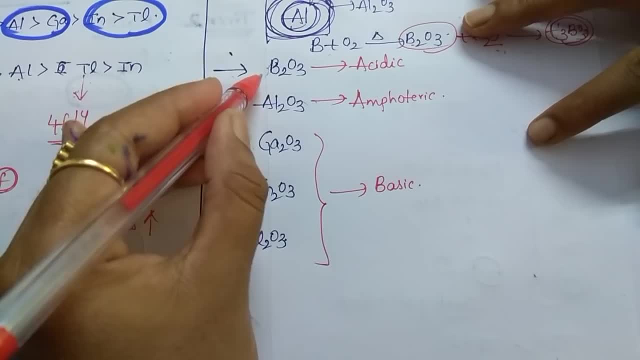 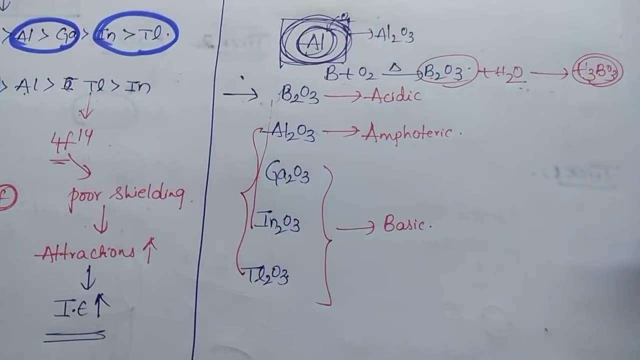 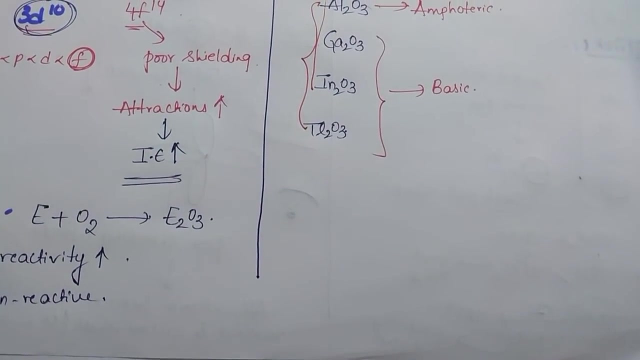 of the following is an acidic oxide? they give these four options. which of the following is an amphoteric oxide? they give these four options. then you should be able to identify which is a acidic, basic and amphoteric, whenever, whenever here i'll discuss, suppose, when the element is reacting with 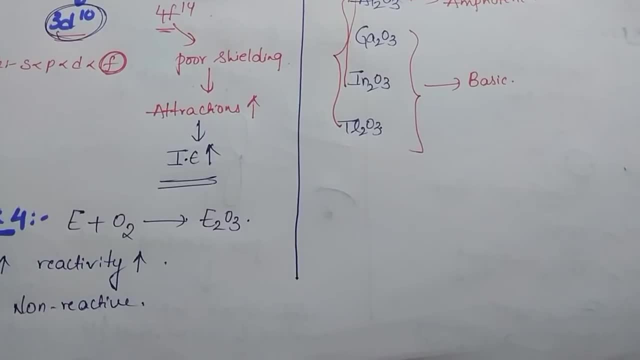 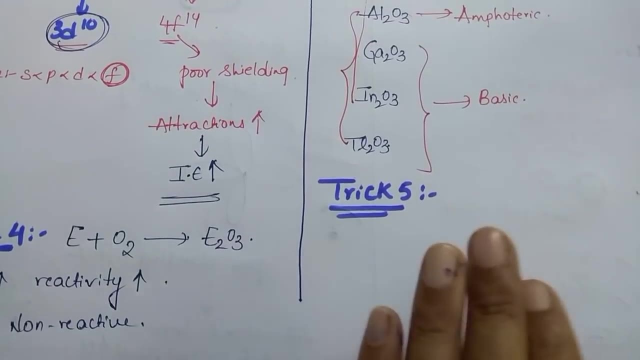 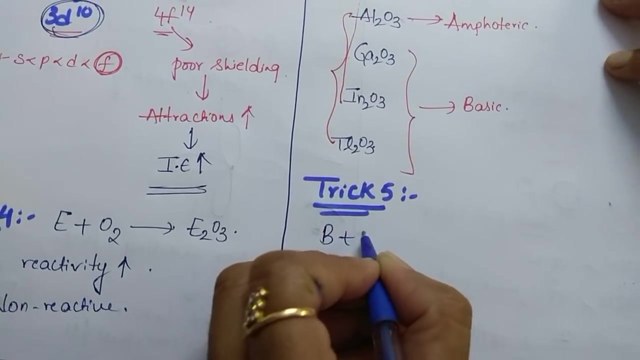 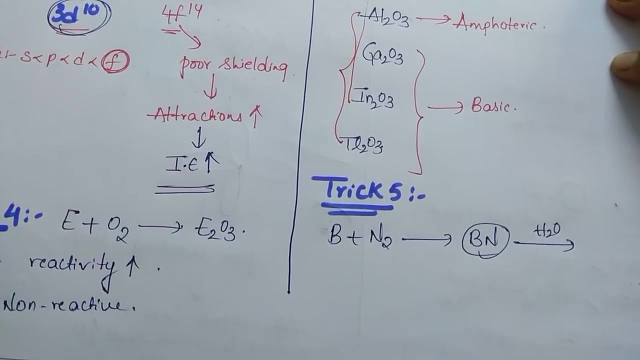 oxygen. you are getting this right. i'll discuss with nitrogen trick number five with this. here i will cover the hydrolysis part, which is very important. suppose boron reacts with oxygen, it forms b2o3. suppose if it reacts with hydrogen it forms boron nitride. this boron nitride, further hydrolysis, is a products. how to do this. 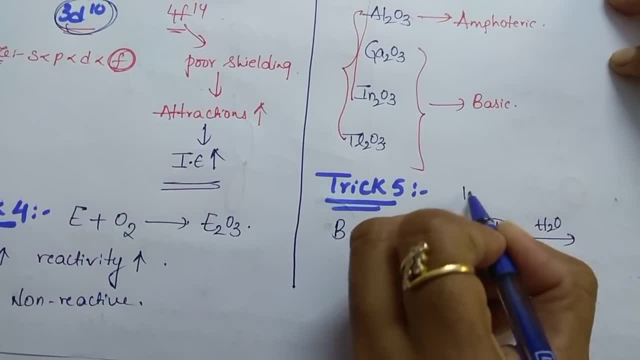 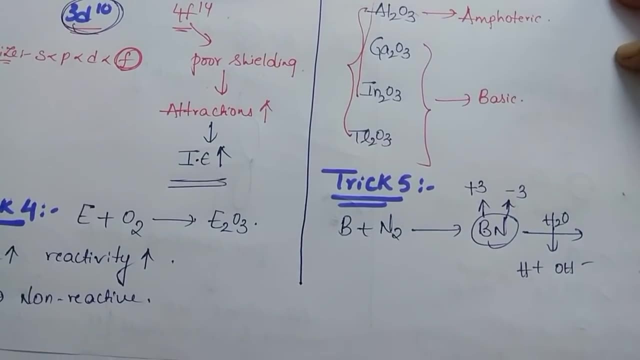 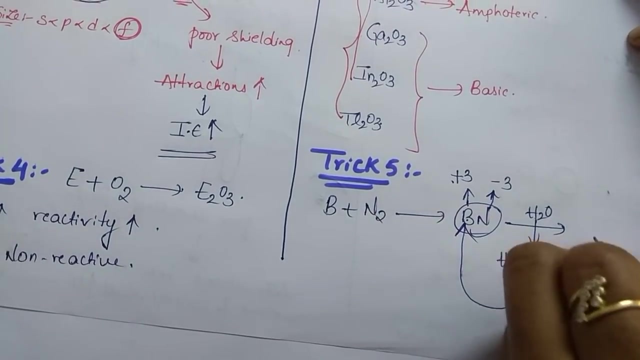 actually in bn boron is in plus three state and nitrogen is in minus three state. if h2o dissociates, it dissociates into h plus and oh minus. so this oh minus goes and attack b3 plus how many- what is the charge? plus three. so it combines with three oh minus and it forms boh thrice and n minus three.